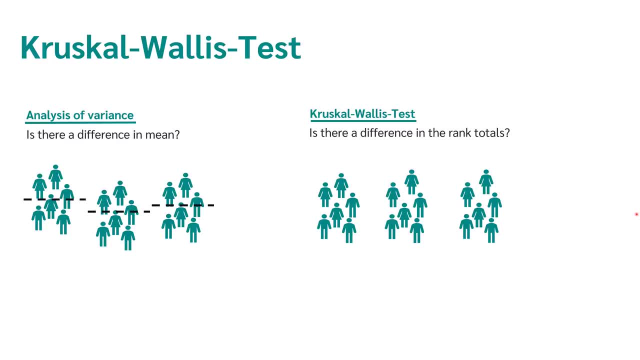 In the Kruskal-Wallis test we do not use the actual measured values, but we sort all people by size and then the person with the smallest value gets the new value or rank. 1. The person with the second smallest value gets rank. 2. The person with the third smallest. 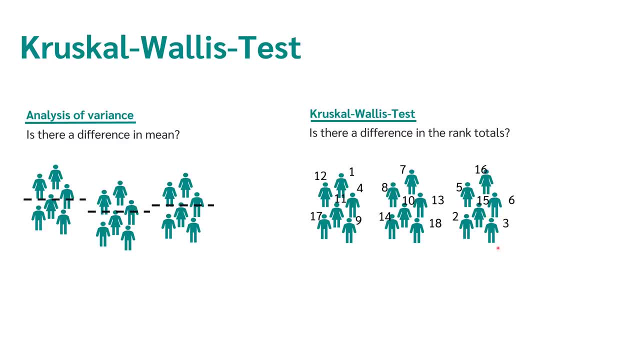 value gets rank 3, and so on and so forth, until each person has been assigned a rank. Now we have assigned a rank to each person and then we can simply add up the ranks from the first group, add up the ranks from the second group and add up the ranks from the third group. 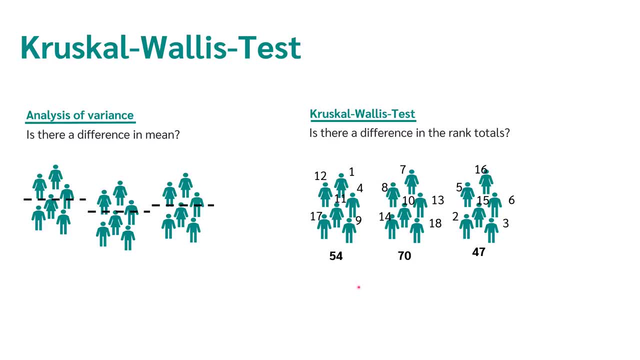 In this case we get a rank sum of 42 for the first group, 70 for the second group and 47 for the third group. The big advantage is that if we do not look at the mean difference but at the rank sum, the data does not show the difference between the main and the second group. The data does not. 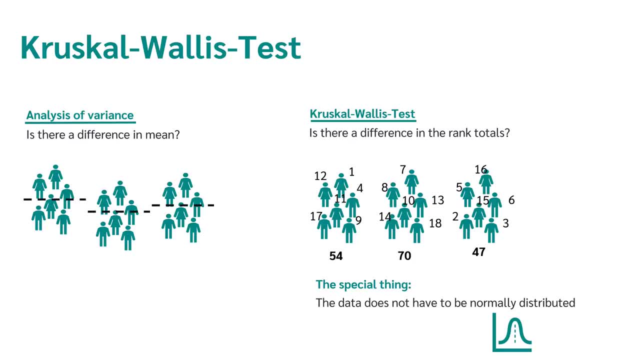 have to be normally distributed When using the Kruskal-Wallis test. our data does not have to satisfy any distributional form and therefore we also don't need it to be normally distributed Before we discuss how the Kruskal-Wallis test is calculated. and don't worry. 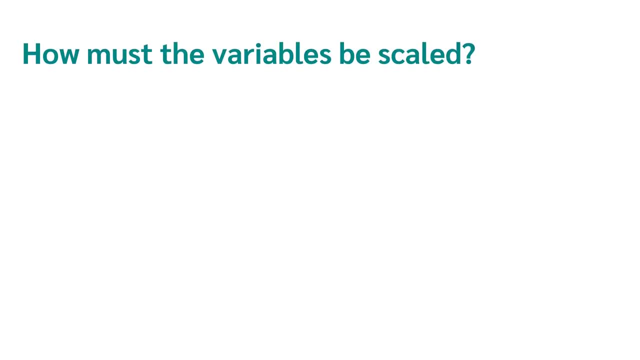 it's really not complicated. we first take a look at the assumptions. When do we use the Kruskal-Wallis test? We use the Kruskal-Wallis test if we have a nominal or ordinal variable with more than two values and a metric variable. 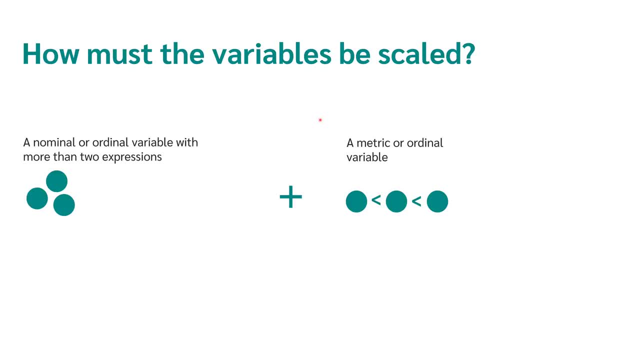 A nominal or ordinal variable with more than two values is, for example, the variable preferred newspaper with the values Washington Post, New York Times, USA Today. It could also be frequency of television viewing, with daily several times a week, rarely, never, A metric. 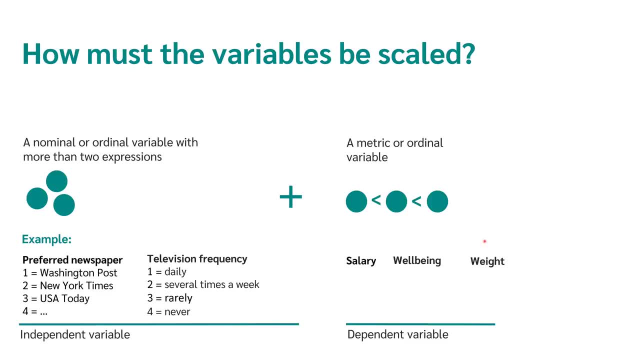 variable is, for example, the sales of a product. If we have a nominal or ordinal variable with more than two values, we also use the Kruskal-Wallis test if we have a nominal or ordinal variable with more than two values and a metric variable. What are the assumptions now? 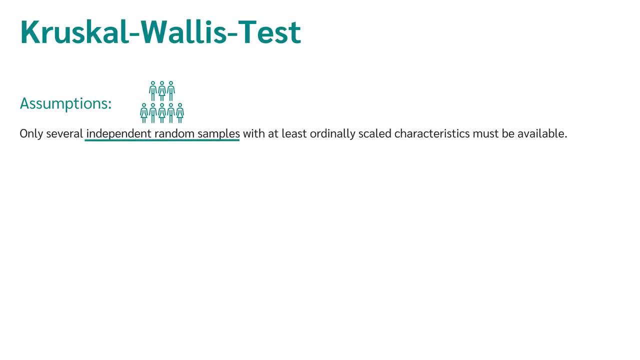 Only several independent random samples with at least ordinarily scaled characteristics must be available. The variables do not have to satisfy a distribution curve, So the null hypothesis is the independent samples all have the same central tendency and therefore come from the same population, Or in other words, 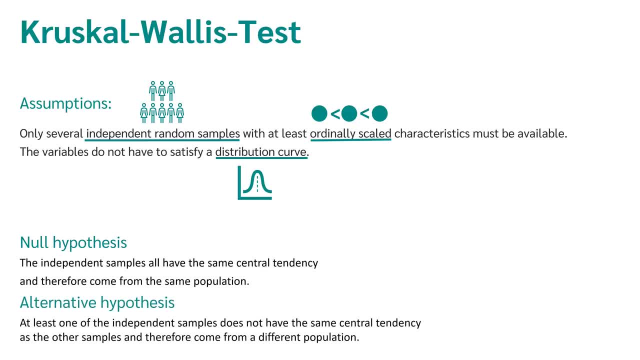 there's no difference in the rank sums, And the alternative hypothesis could be: at least one of the independent samples does not have the same central tendency as the other samples and therefore comes from a different population. Or, to say it in other words, again, at least one group differs in rank sums. 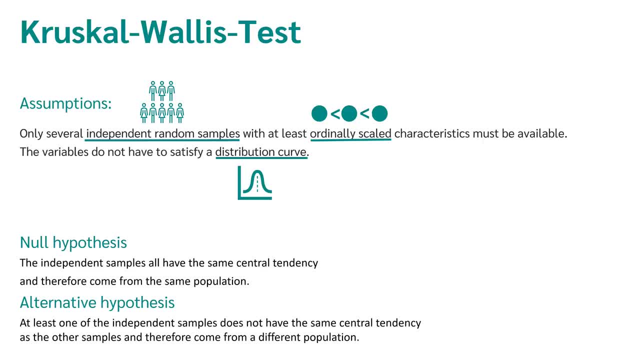 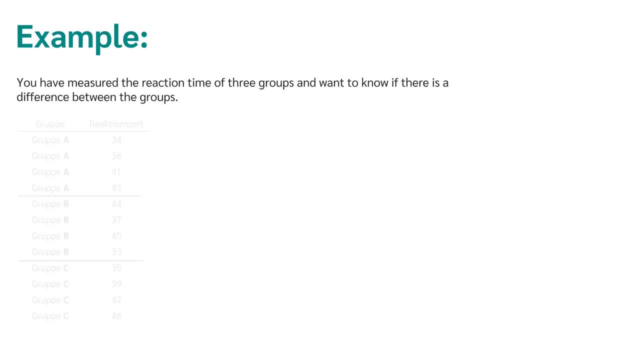 So the next question is: how do we calculate a Kruskal-Wallis test? It's not difficult. Let's say you have measured the reaction time of three groups- group A, group B and group C- And now you want to know if there's a difference between the groups in terms of. 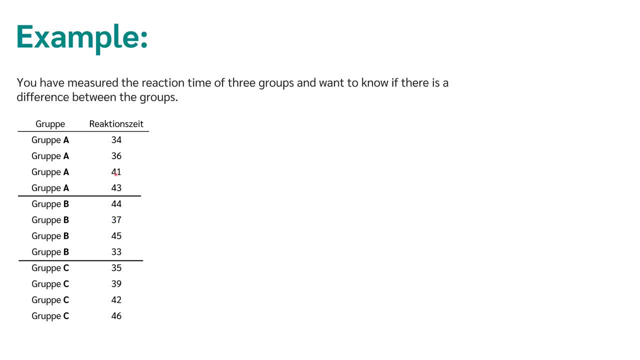 reaction time. Let's say you have written down the measured reaction time in a table. Let's just assume that the data is not normally distributed and therefore you have to use the Kruskal-Wallis test. So then our null hypothesis is that there is no difference between the groups. 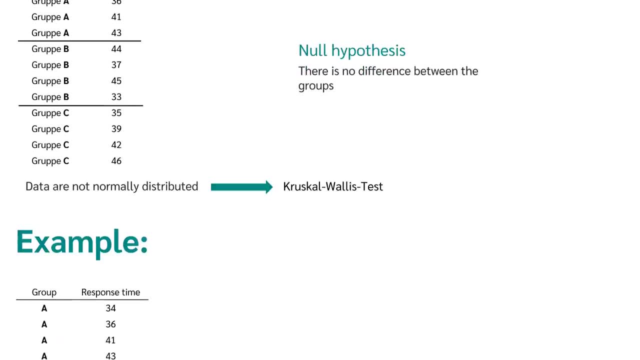 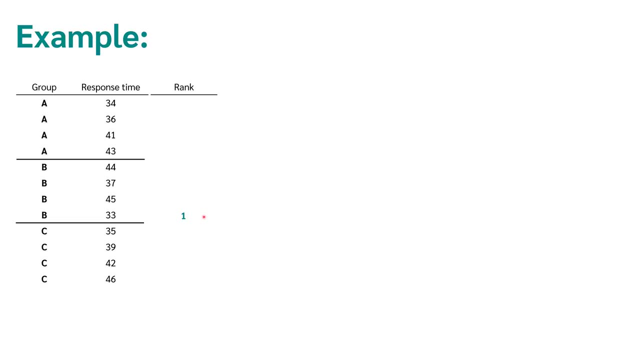 And we're going to test that right now. First, we assign a rank to each person. This is the smallest value, so this person gets rank 1.. This is the second smallest value, so this person gets rank 2.. And we do this now for all people. 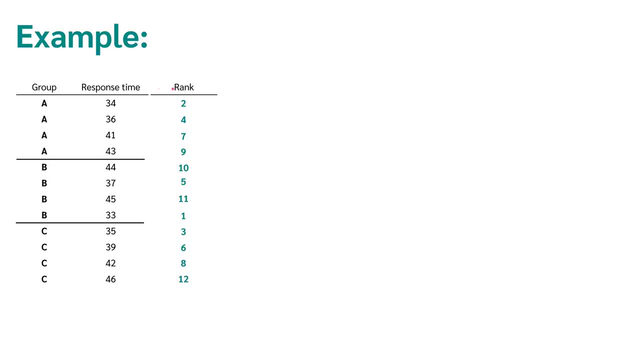 If the groups have no influence on reaction time, the ranks should actually be distributed purely randomly. In a second step We now calculate the rank sum and the mean rank sum. For the first group, the rank sum is 2 plus 4 plus 7 plus 9, which is equal to 22.. And we have 4 people in the group. so the mean rank sum is 22 divided by 4, which equals 5.5.. Now we do the same for the second group. Here we get a rank sum of 27 and the mean rank sum of 6.75. 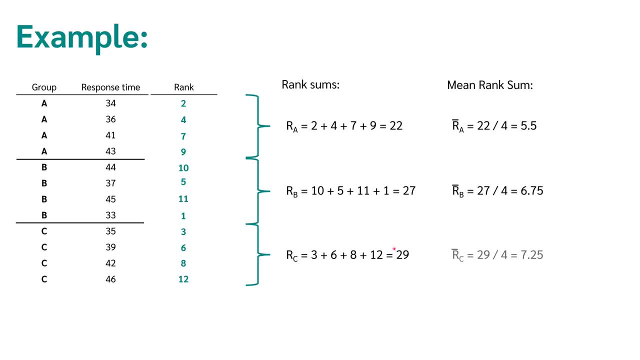 Let's see. And for the third group, we get a rank sum of 29 and the mean rank sum of 7.25.. Now we can calculate the expected value of the rank sums. The expected value, if there is no difference in the groups, would be that each group would. 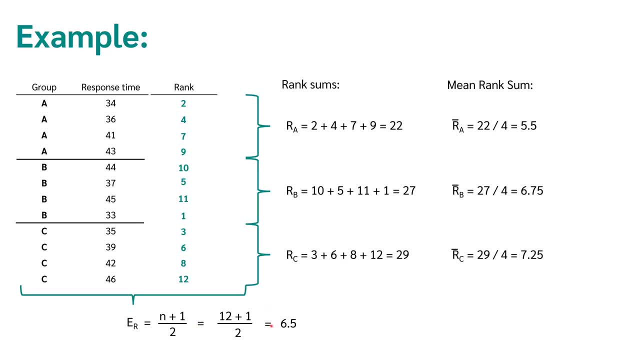 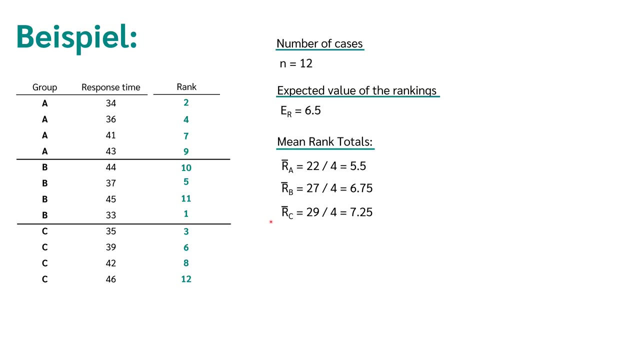 have a rank sum of 6.5.. We've now almost got everything we need. We interviewed 12 people, so the number of cases is 12.. The expected value of the ranks is 6.5.. We've also calculated the mean rank sums of the individual groups. 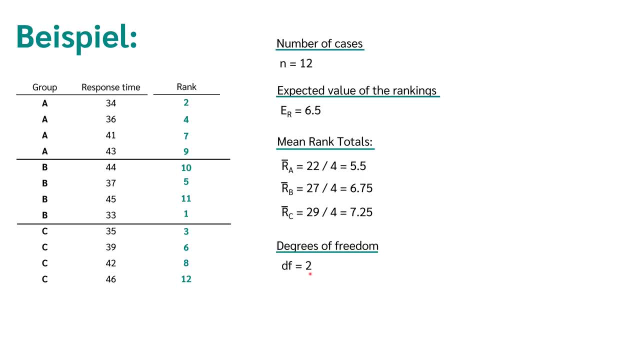 The degrees of freedom, in our case are 2, and these are simply given by the number of groups minus 1, which makes 3 minus 1.. Last, we need the variance. The variance of ranks is given by n to the power of 2 minus 1 divided by 12.. 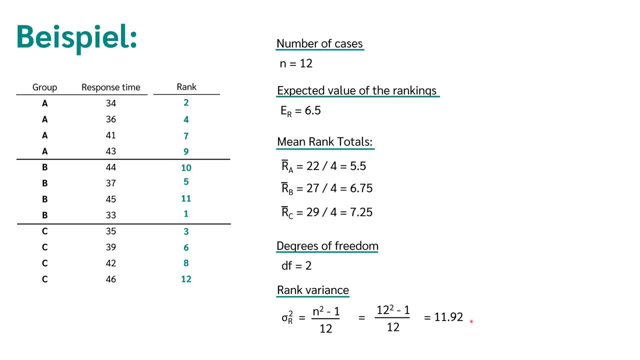 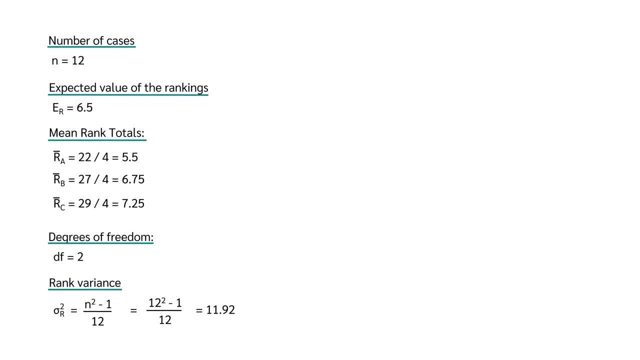 n is again the number of people, so 12.. So we get a variance of 11.92.. That's it. Now we've got everything we need. With these values, we can now calculate our test value h. The test statistic. h corresponds to the g-square value and is given by this formula: 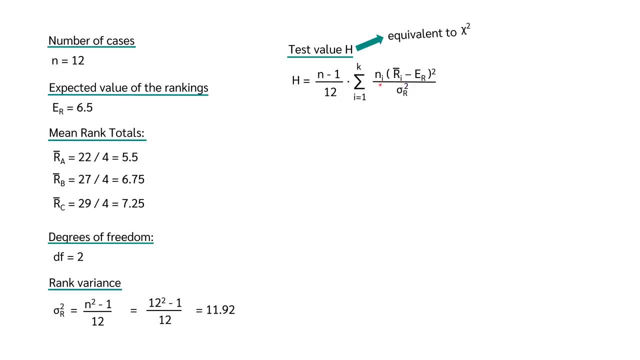 n is the number of cases, r-bar is the mean rank sum of the individual groups and er is the expected value of the ranks. Sigma squared is the variance of the ranks. In our case, r-bar is the variance of the ranks. 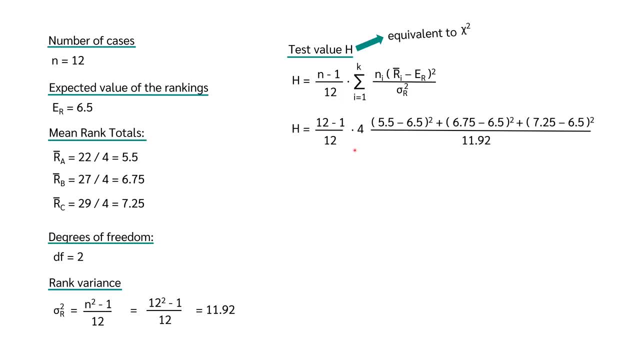 In our case, the number of cases is 12.. We always have 4 people per group so we can pull out the ne. 5.5 is the mean rank of group A, 6.75 is the mean rank of group B and 7.25 is the mean. 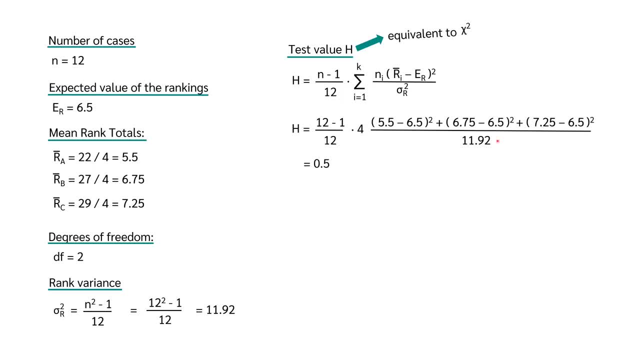 rank of group C. This gives us a rounded h value of 0.5.. As we just said, this value corresponds to the g-square value. So now we can easily read the critical g-square value in the table of critical g-square values. 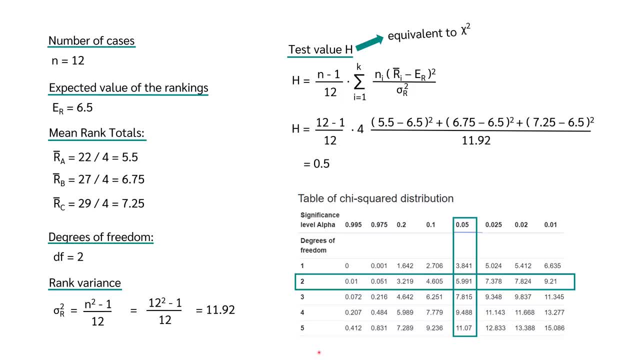 You find this table on datatabnet. We have 2 degrees of freedom and if we assume that we have a significance level of 0.05, we get a critical g-square value of 5.991.. So of course, our value is smaller than the critical g-square value. 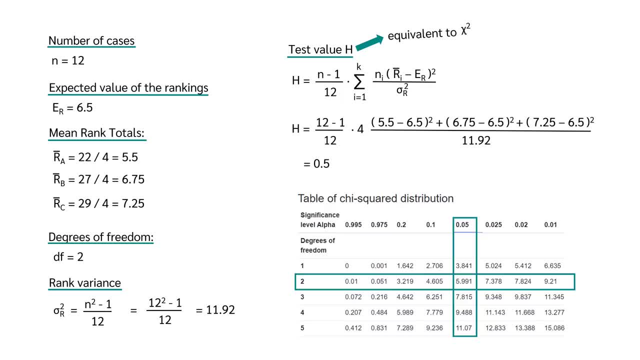 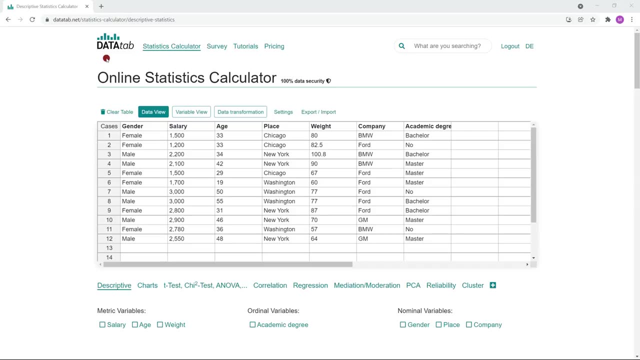 And so, based on our example data, the Nihil hypothesis is retained. And now I will show you how you can easily calculate the Kruskal-Wallis test online with datatab. In order to do this, you simply visit datatabnet. you will find a link in the video description.